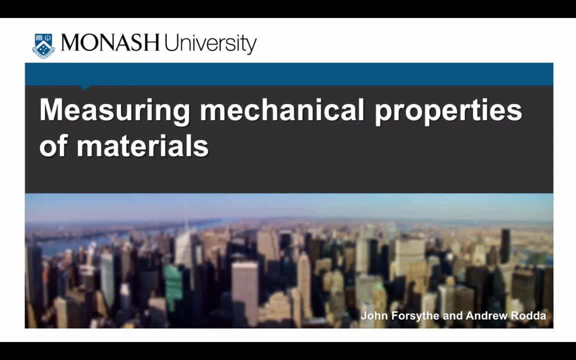 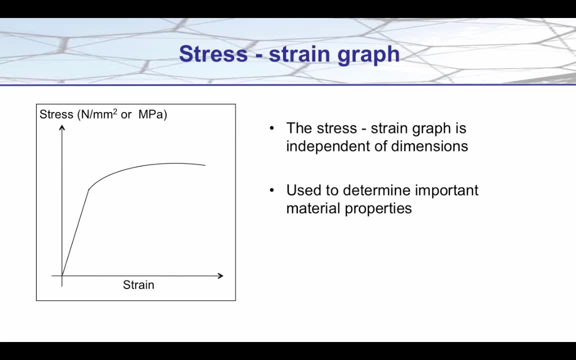 Hello, my name is John Forsyth and in this lecture I will be covering the measurement of mechanical properties of materials. In the previous online lecture we performed a tensile test on a material specimen and obtained the resultant stress versus strain plot. These plots are independent of the 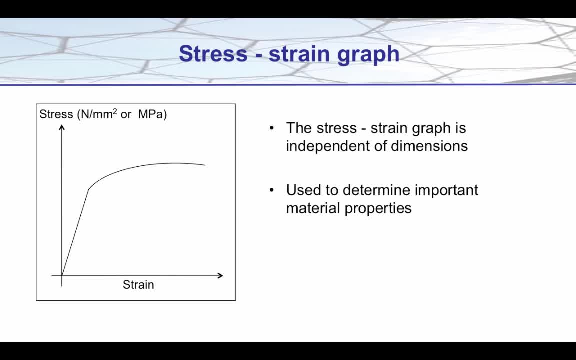 material specimen dimensions and allows us to compare the tensile response of different types of materials. We saw that the plot has two different regions. We have the elastic region, where all deformation is recoverable, and we have the plastic region where we have non-recoverable deformation. However, 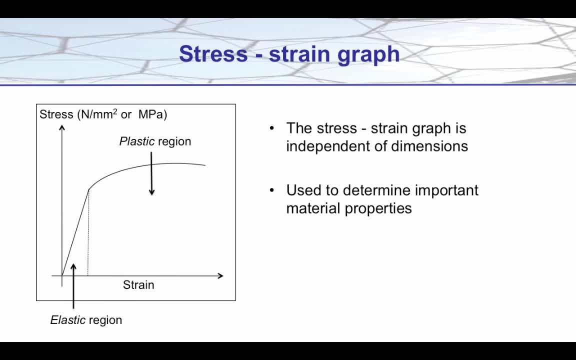 these plots contain a wealth of information, such as important mechanical properties, and in this lecture we're going to take a closer look at the stress versus strain plot. We will learn how to interpret the plots and how to extract very important mechanical properties of materials which can be used in design. Now the first. 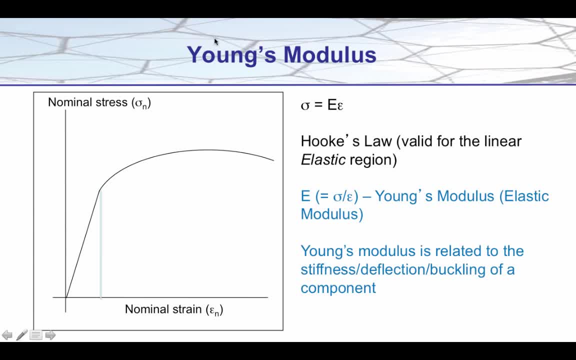 material property that we're going to look at is the Young's modulus. It's a very important material property. If we have a look at the elastic region, we see that the stress and the strain are directly proportional and if we take the equation of that line, it's given by hooks. 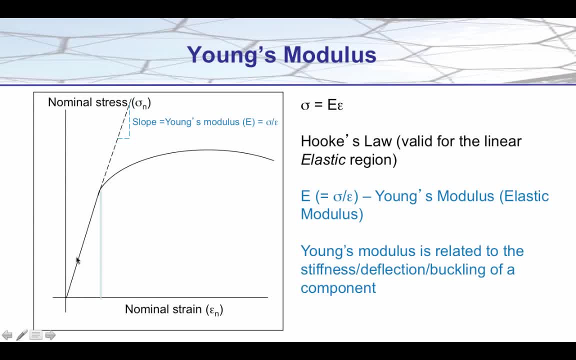 Hooks law, which is valid only within this elastic region. So hooks law states that the stress is directly proportional to the strain multiplied by the modulus. and the modulus is a material property, So different materials have different Young's modulus. This is a very important parameter as it determines how 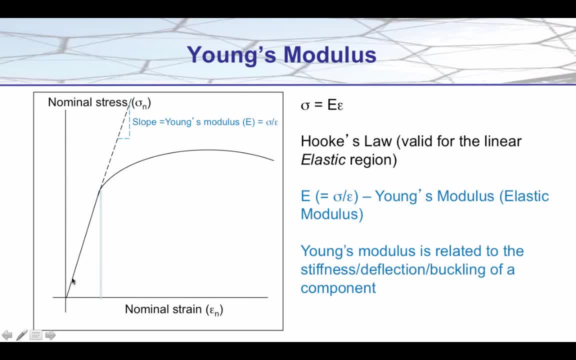 much deformation will occur within the elastic region. So materials with a high modulus will undergo less elongation or strain for a given stress. or conversely, for a given amount of strain, a higher modulus material experience a higher stress. The Young's modulus is critical in engineering as it 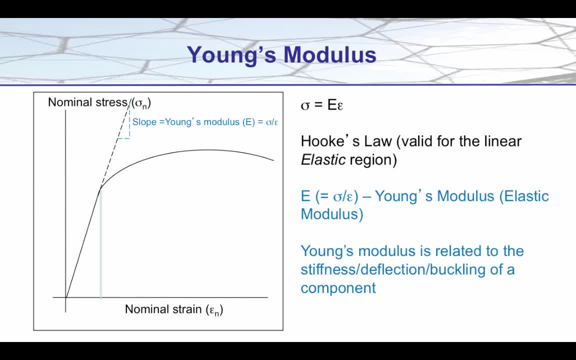 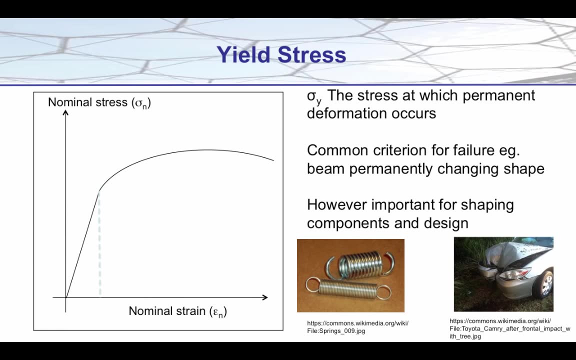 is related to the stiffness of the component, how much deflection it undergoes and the buckling of the component if it's under compression. It all depends on the type of loading imposed on the member. The stress at which we move from the elastic region to the plastic region is 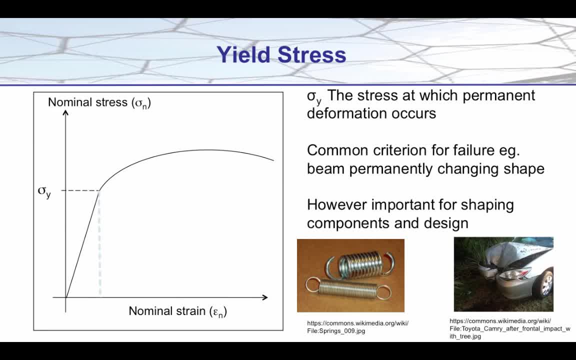 known as the yield stress or yield strength of the material. At this point there is non-recoverable or permanent deformation in the specimen. Often in structural engineering, components are designed so that they only operate in the elastic region, as permanent deformation is unwanted, For example, a 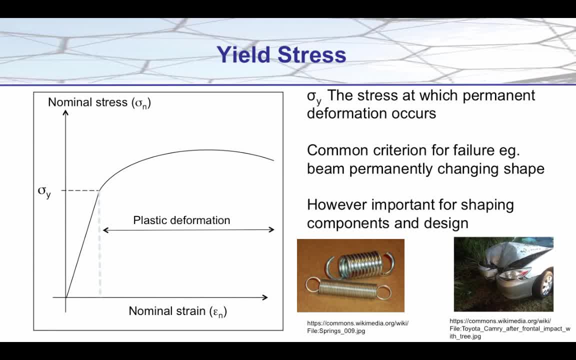 beam that has permanently deformed will often need to be removed. However, plastic deformation is important when we want to start to permanently shape a component. Let's say, make a wire into a spring requires plastic deformation, and also car bodies are now designed to have a significant crumple. 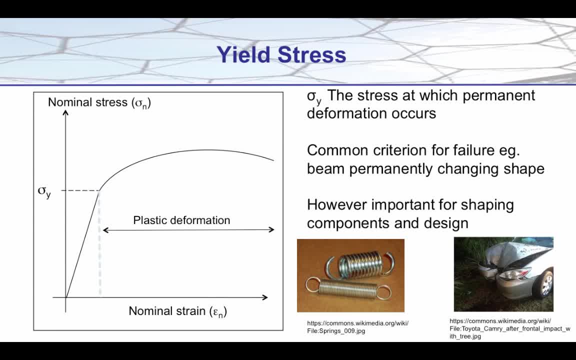 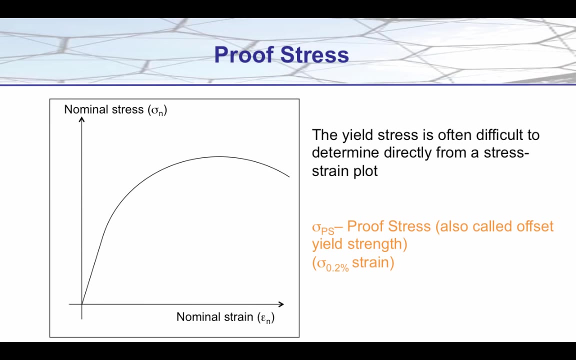 zone. Upon impact, the car panels undergo severe plastic deformation, which absorbs crash energy and protects the occupants of the vehicle. The yield stress and plastic deformation are therefore important to consider when selecting materials for engineering applications. Very often it is difficult to definitively define the yield stress of a stress-strain curve, as 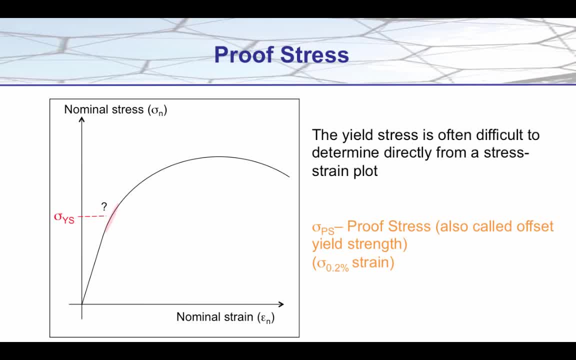 it is difficult to locate the transition from the linear elastic region to the nonlinear plastic region. To get around this problem, we use the proof stress Here. we move out from the origin- a nominal 0.2% or 0.002 strain and draw a. 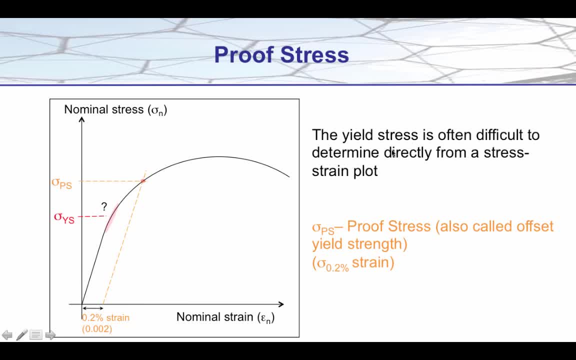 line parallel to the initial slope. where the line intersects the curve is known as the 0.2% proof stress. Now, just be aware that sometimes engineers use, instead of 0.2%, they use 0.1%. It doesn't really matter what you use, just as long as 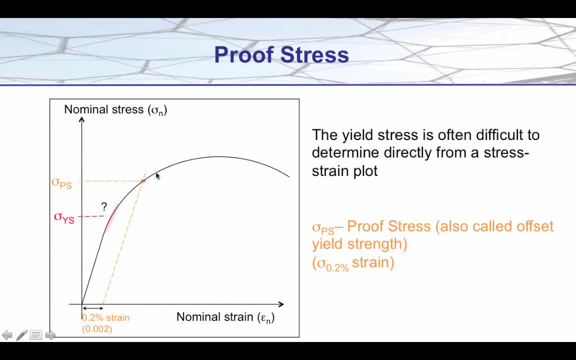 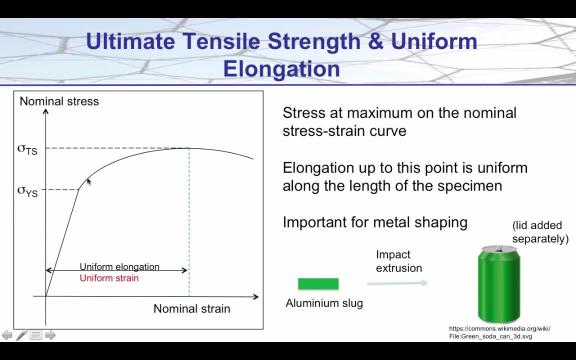 you indicate what you are using to determine your proof stress. So within the plastic region, the engineering stress increases up to a maximum value known as the tensile strength, or sometimes the ultimate tensile strength. So this is the maximum in the curve up here. This is the maximum stress that can be sustained by. 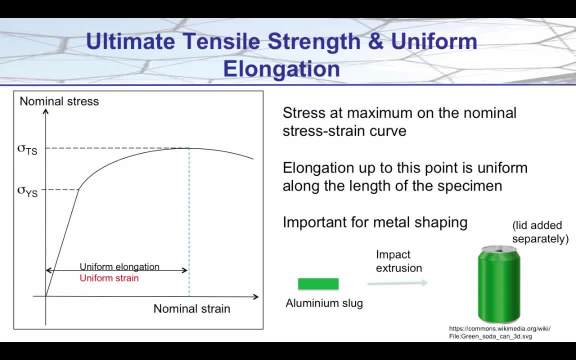 a structure without fracture occurring. Now, up until this point, elongation has been stable, resulting in uniform elongation along the length of the sample. So all along here has been uniform strain, Uniform strain and uniform elongation is very important in processing and shaping For. 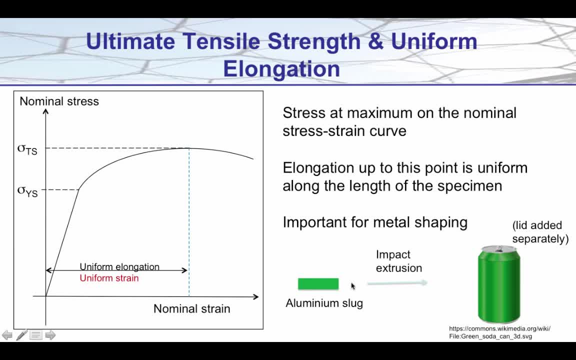 example, if we were to make an aluminium can. the way that they do that is they get an aluminium sample, an aluminium slug, and undergo a process called impact extrusion, which draws out the slug into the final shape of that can. Now the process relies on uniform elongation of the aluminium slug so that the wall thicknesses 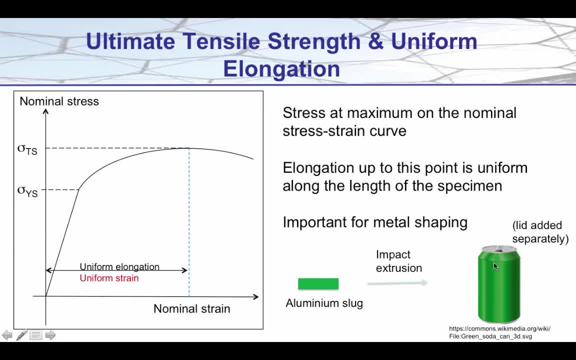 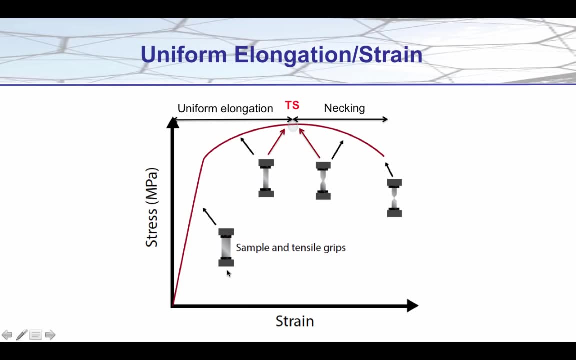 are uniform along its length. Note that the lid on the beverage can is actually made out of a different type of material and is added to the can in a separate process. Now in this plot we see what will happen to a sample as it undergoes a tensile test. Now in the elastic region it will 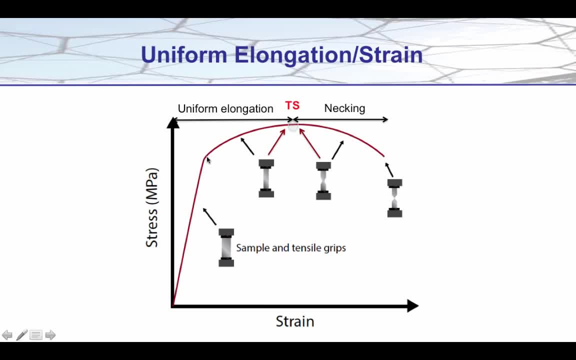 elongate uniformly and as we go past the yield stress it will continue to uniformly elongate. so it's changing dimensions evenly across the entire sample up to the point of the ultimate tensile strength. As we move past the ultimate tensile strength- something very interesting- 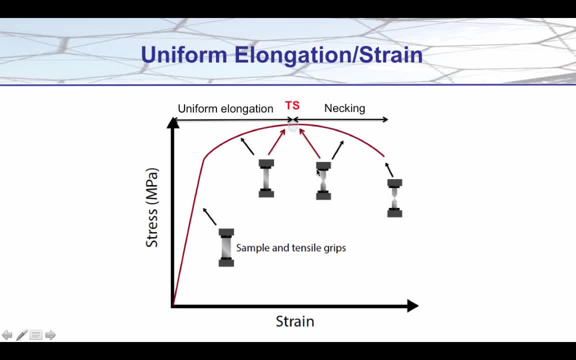 happens and we see that all deformation is now localized, with the material width, in a particular region and that now causes it to form a neck. Now this process is called necking, and this will occur all the way up to the point of fracture, and fracture will occur in the neck region. 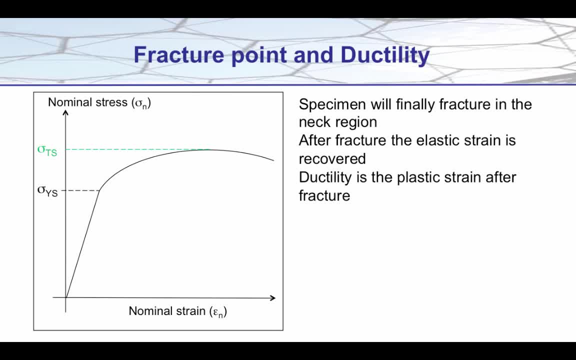 If we maintain a stress past the tensile strength of the material, fracture will occur within the neck region. The fracture point is of little practical importance in structural engineering as we are more interested in the yield strength and the tensile strength of the material in the design process. 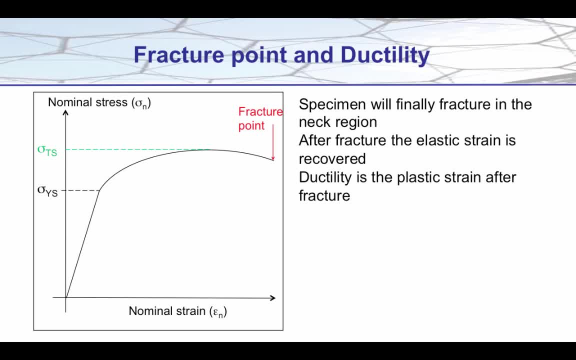 In other words, we do not want to go past the tensile strength where there is significant and localised plastic deformation. However, something interesting occurs just as the specimen fractures. When it breaks, it actually snaps back a little bit and the sample becomes smaller. 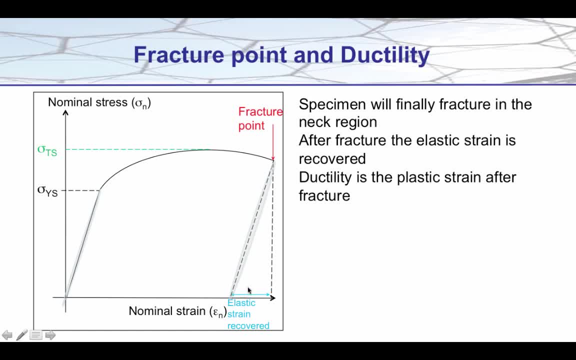 The elastic strain which originally occurred right at the start of the experiment is recovered. The amount of plastic strain that occurs in the sample after fracture is known as the ductility. The ductility can be expressed quantitatively as either a percentage elongation. 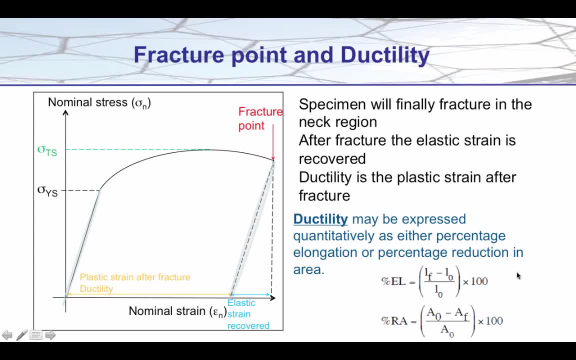 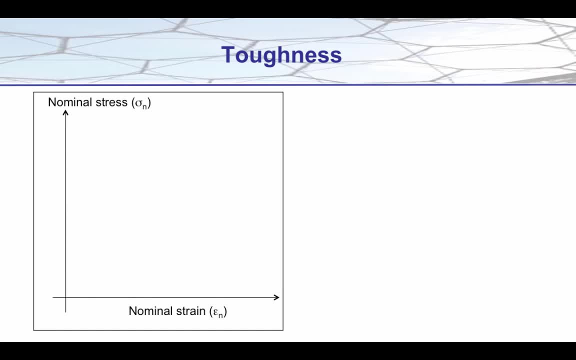 or percentage reduction in the area given by these experiments. The final material property that we are going to look at is called the toughness. I'm sure you've heard of the term toughness, but don't know exactly what it is. If we did a tensile test on a specimen and saw a response looking like this: 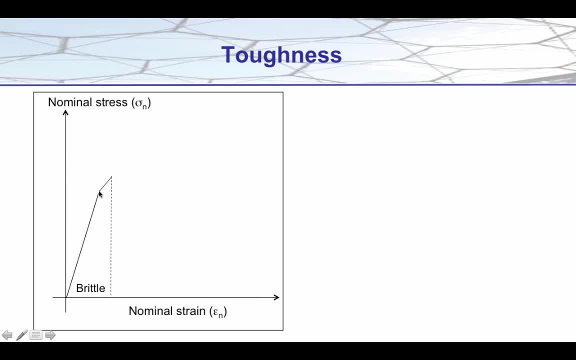 where we have the elastic region. it hits its yield point but doesn't plastically deform very much. So as soon as it hits its yield point it breaks. We would call this sample a very brittle material because it doesn't undergo very much plastic deformation. 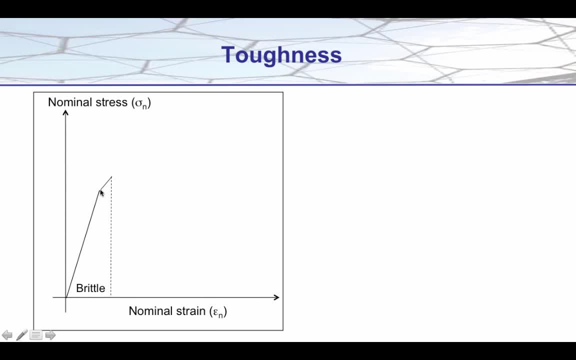 It doesn't undergo very much plastic deformation. An example of material that would be like this would be glass, or, in fact, your spaghetti that you're using to make your spaghetti bridge. If we had another sample, exactly the same modulus, exactly the same yield, stress, but undergoes a lot of plastic deformation. 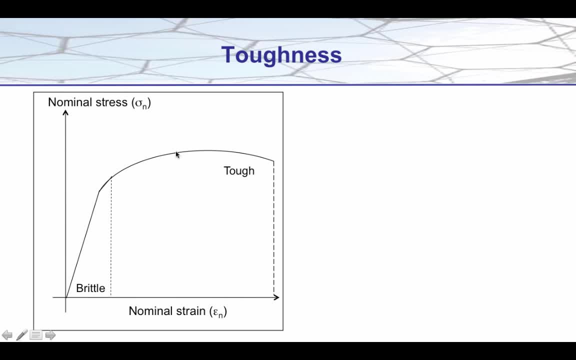 up to the point here where it fractures, this would be a comparatively tougher material. The toughness is defined as the amount of work done per unit. The toughness is defined as the amount of work done per unit. The toughness is defined as the amount of work done per unit. 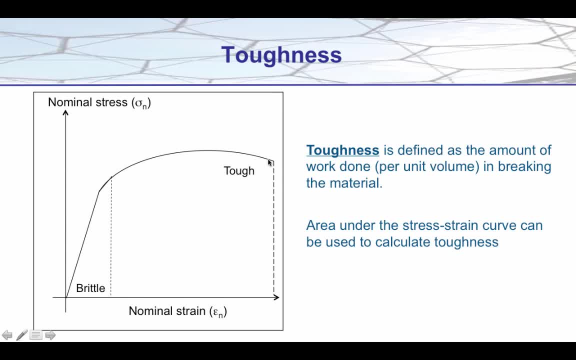 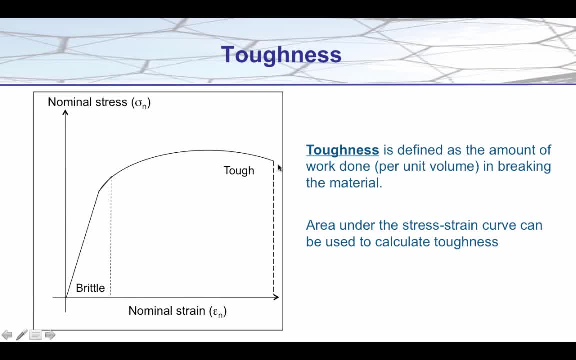 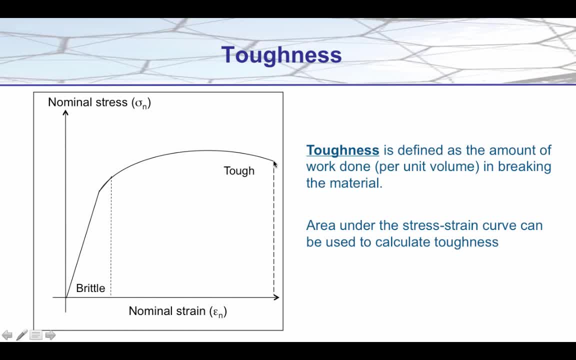